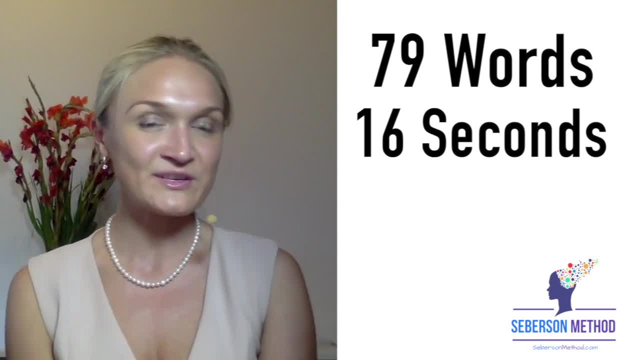 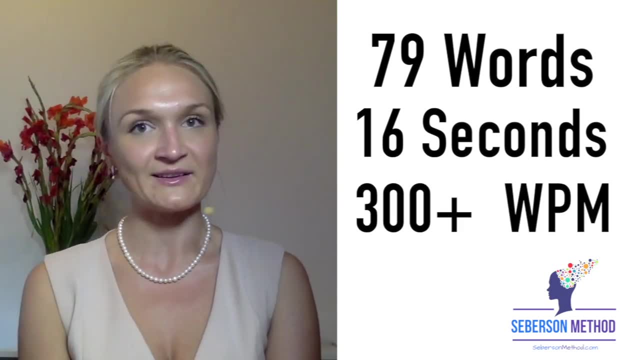 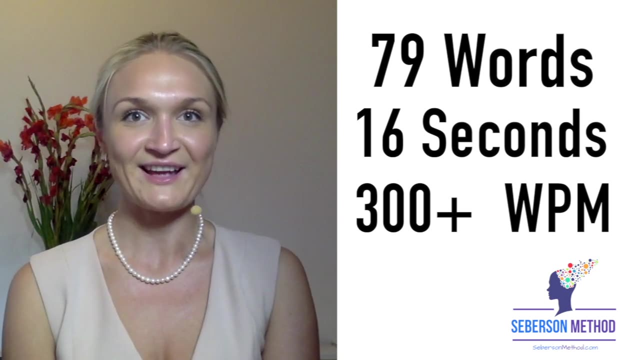 16. And in order to get through the 79 words, you will have to maintain a speed of 300 words per minute, or faster. Again, if you feel like that's a little bit too fast for you, feel free to pause me, but don't give yourself more than 30 seconds. It's not about you memorizing the 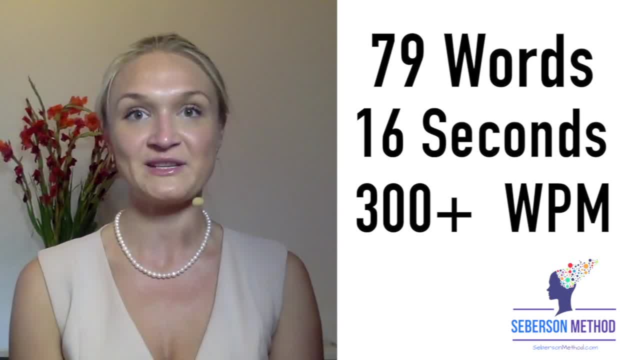 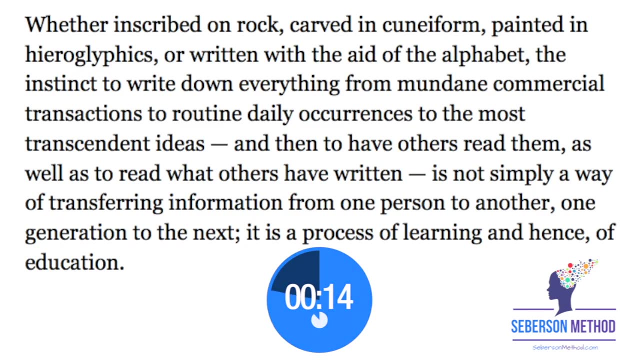 sentence. It's about you understanding what the sentence is saying. Reading comprehension is not about memorization. Reading comprehension is about making meaning from text. Ready, set, go, Welcome back. What did you guys think? Take out your blank sheet of paper and write down the. 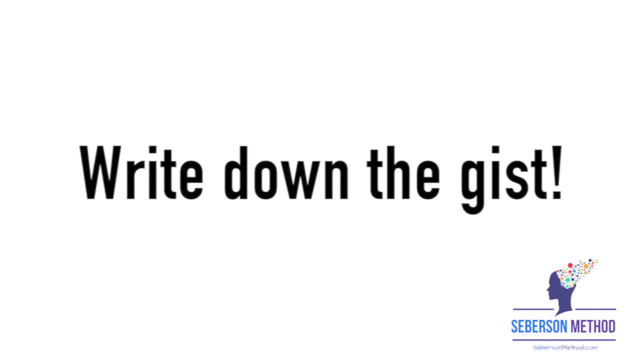 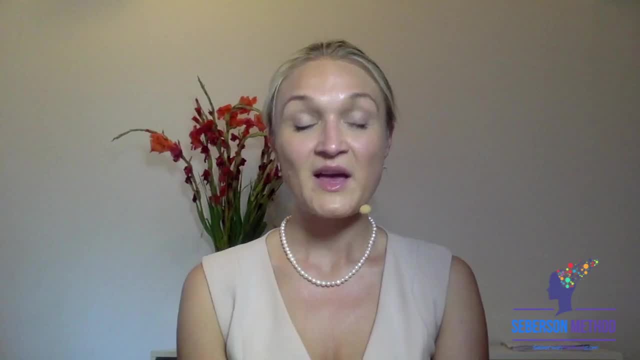 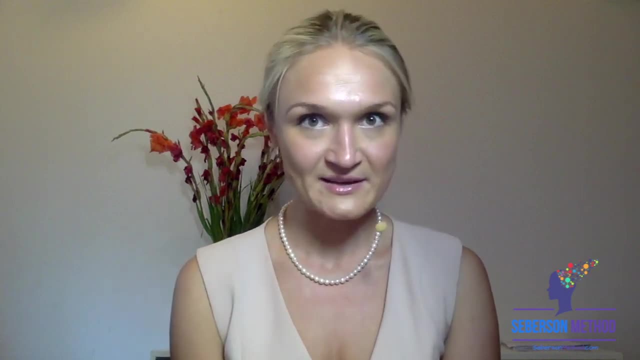 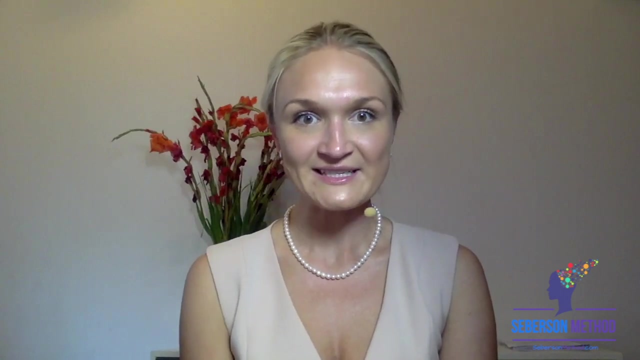 gist of this sentence. Who did what? What's your subject? What's your verb? What's your compliment? What's your additional phrase? If you had something along the lines of the instinct to write things down, that's my subject. the instinct to write things down is not, that's my verb. this is a to be verb, is not? 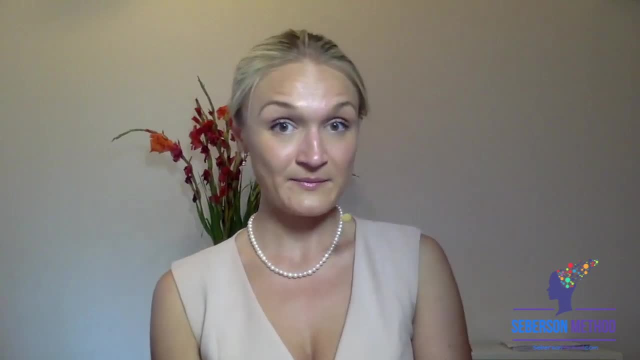 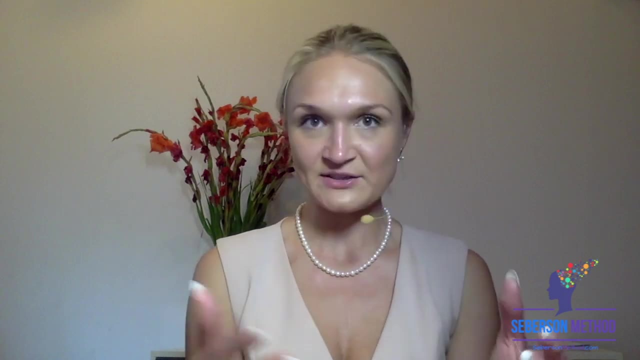 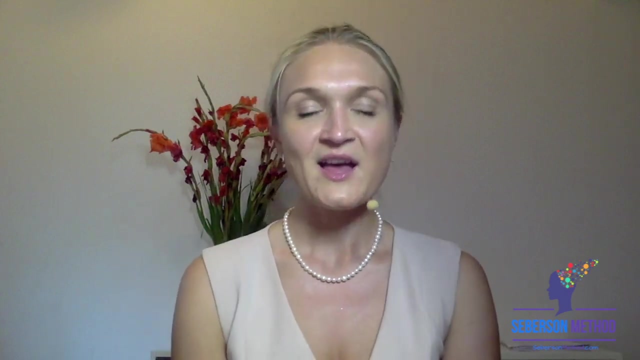 simply a way of transferring information, but it's a way of learning and education. So the instinct to write things down is not a way of transferring information, but it's a way of learning. If you had something similar, great job. But if you thought that the subject was the, 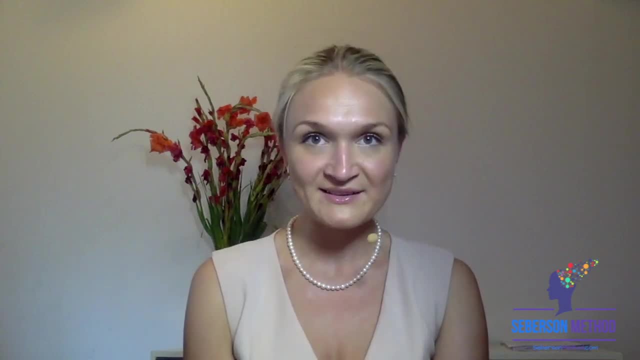 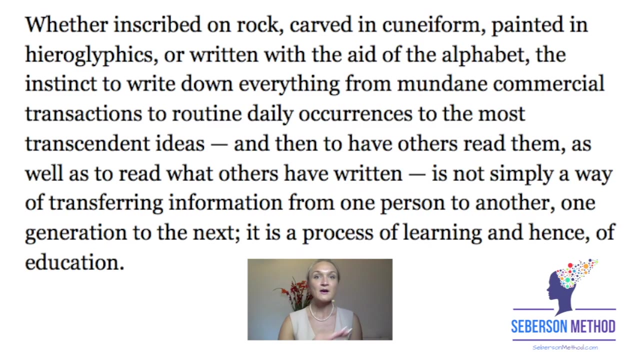 hieroglyphs, the cuneiforms or the alphabet. let me show you what an advanced Jackie would do and how she would approach the sentence. First and foremost, she would look at the sentence and she definitely doesn't want to go to audio. She first notices the word weather. Weather is. 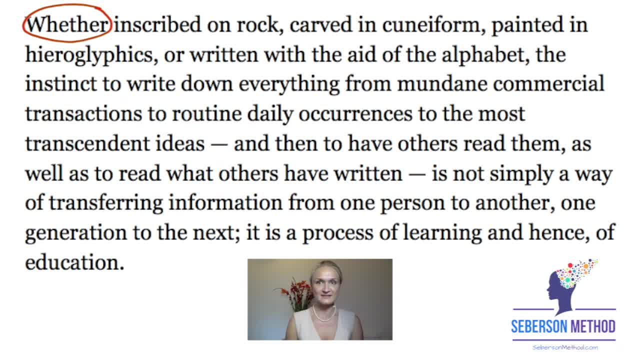 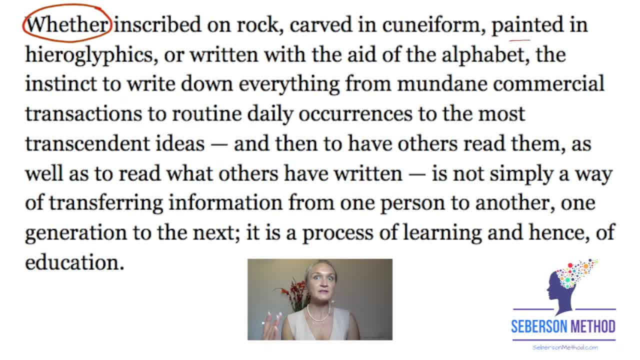 this is going to be an opener. She immediately knows that this is an advanced sentence structure that actually expanded in the beginning, So she's not even going to look for her subject in here. They're inscribed on rock And she also knows that weather is a paired conjunction. It's weather. 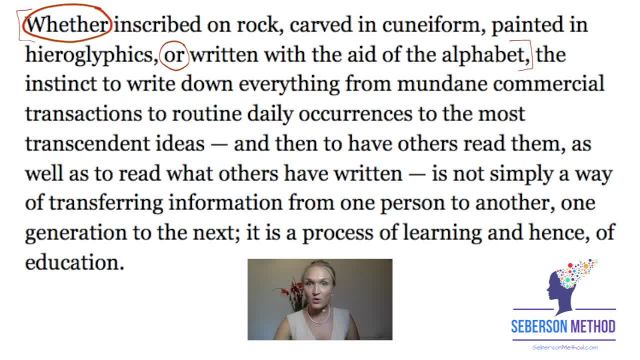 or. So Jackie's going to scan all the way through to the word or and then wait for the comma. And right after the comma, right here, she's going to be expecting her subject. And she gets super lucky. She finds it the instinct. And then she starts looking for her corresponding verb or her. 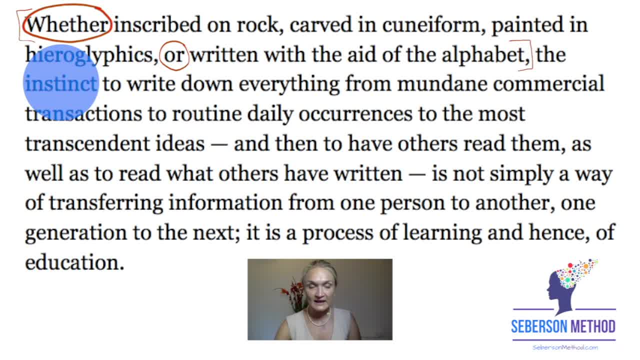 conjugated verb. She begins to scan, She notices that this is a verb, And then she starts looking for the verb by various innexplanatory terminologies. She's going to look for the verb from, And then she removes the verb from verb one, And then I'm. 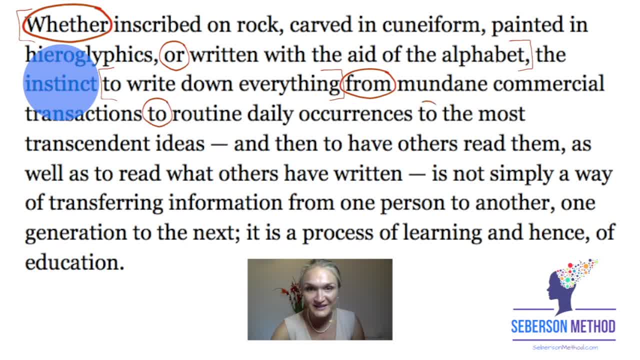 going to go back to that verb verb form. in case you didn't notice, She is going to go over that verb verb at the top And she finds how to use a verb // from verb verb in thehooting use to make a. 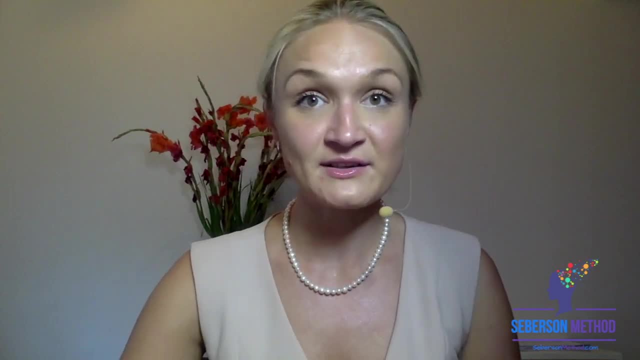 verb that replaces verb. And then she has to sort ofjährally enough to say: the verb is a verb, verb as they are an addition, Which I think is kind of. It also says that a verb is aea in a sentence when a verb is. 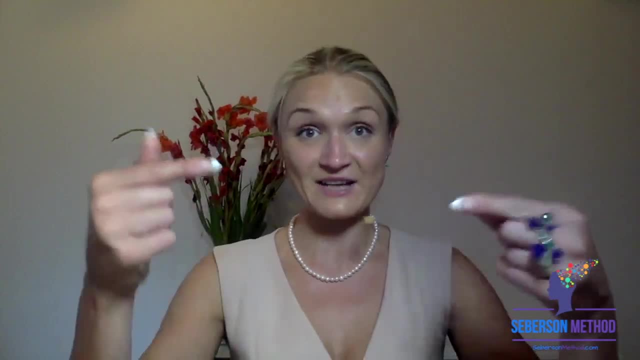 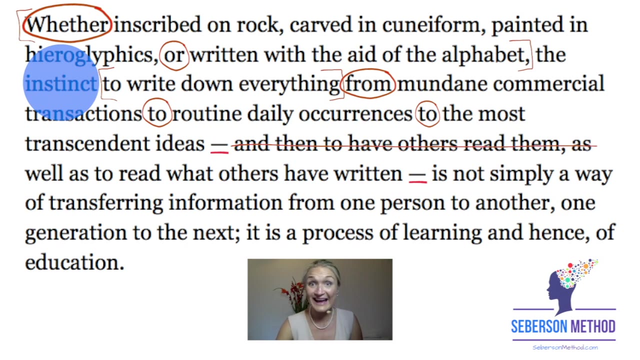 Гê고드 Gem. Variable verbeal phrase: the. she sees preposition from, And then she knows that a proposition from is usually a paired. you remember that something that's offset by dashes on both sides is a non-essential detail. So she is going to miss all of this. She hasn't found her verb yet. Where is it? Here it is. 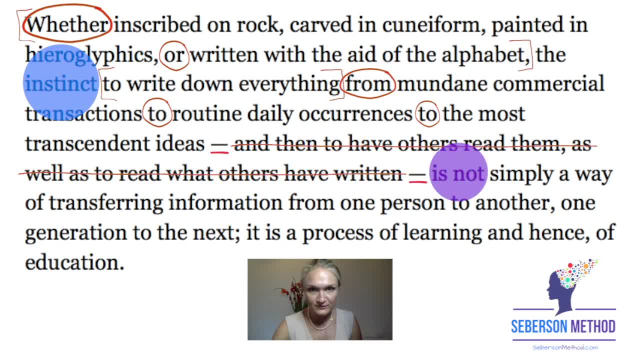 She just found it on one, two, three, four, five. on the sixth line, towards the end of the sixth line of the sentence. So do you see how much they have inserted between the subject and a verb? This is a very complex sentence structure. That's something you will see on the SAT. 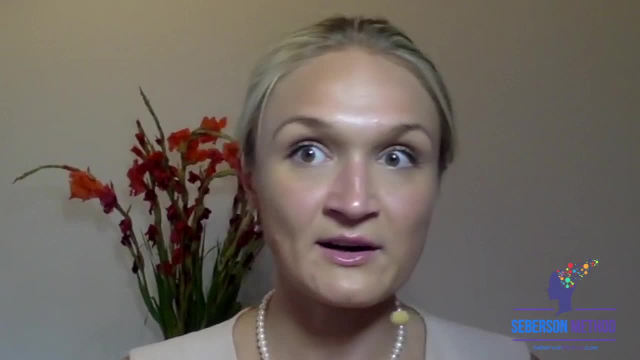 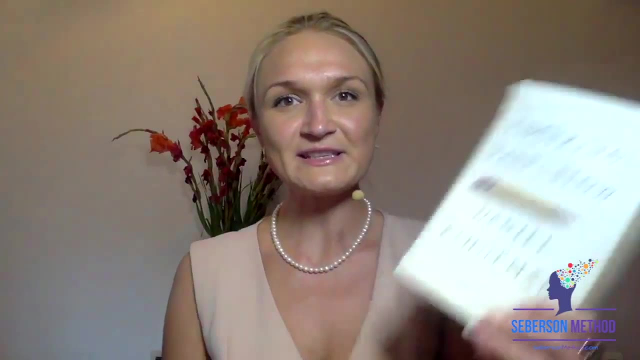 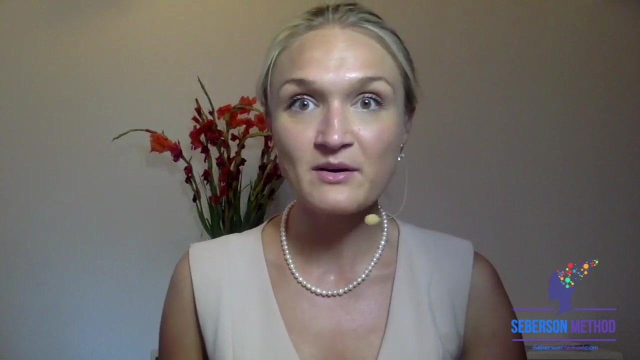 This is a bit too complex for the PSAT And if you're a reader then you would probably see it in the New Yorker or maybe a publication. Actually, this guy, Daniel Kahneman. he loves to use these sentence structures And therefore a lot of people have found his book really interesting. 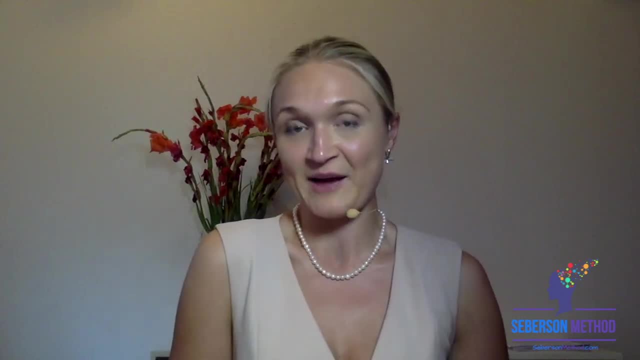 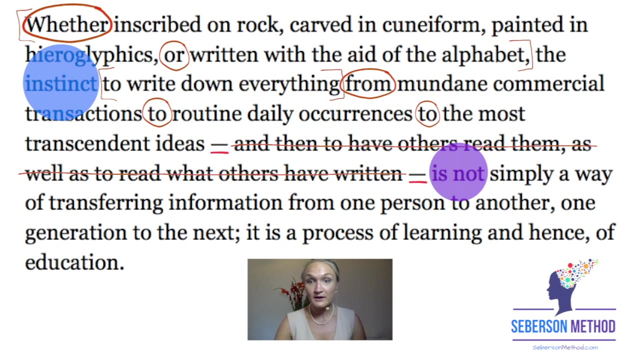 but really tough to read. He doesn't use elevated vocabulary sentence structure, But let me move on. So Jackie's going to find her verb and then she's going to continue scanning and she's going to see something really important. She's going to see a semicolon. 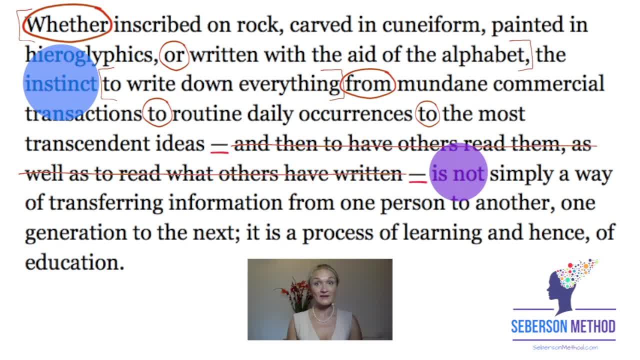 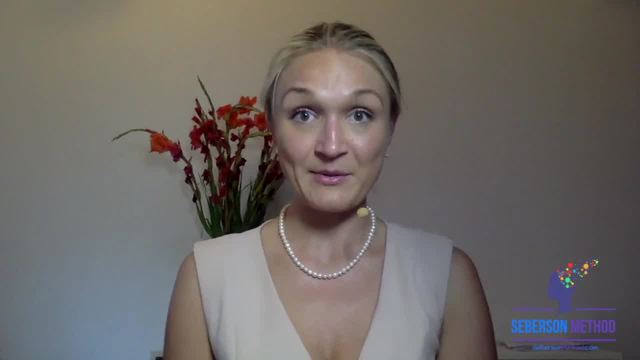 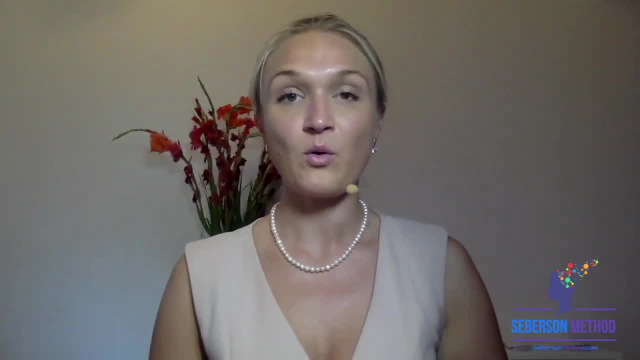 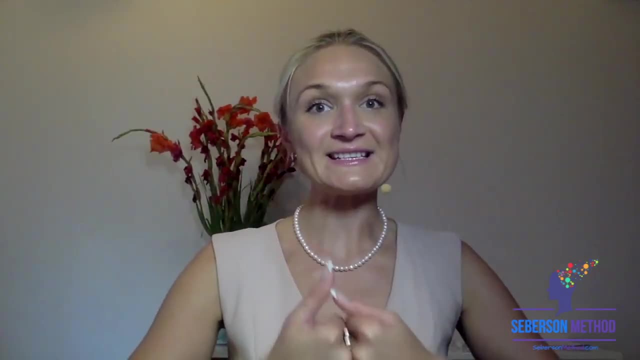 Semicolon is a clear sign to Jackie that this is a compound sentence. Remember, when we were talking about decoding, I was talking about compound words. Compound words consist of a two parts, like backpack, or like background, or everybody or lightheaded. That means this. 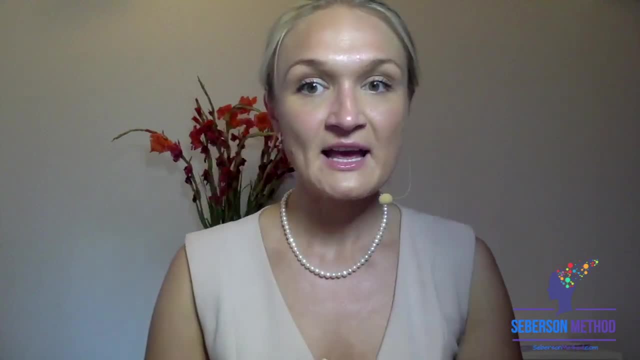 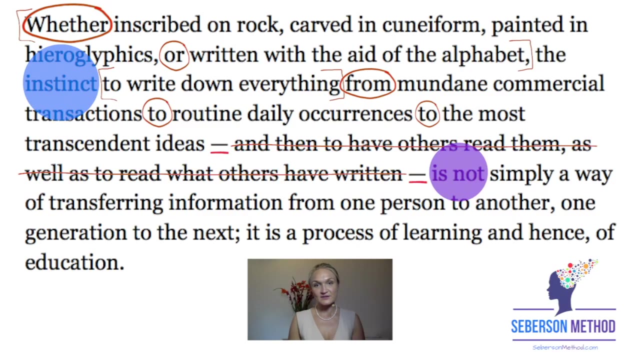 word has two distinct parts. What Jackie quickly realizes is there are two distinct ideas in the sentence. There is one idea that is communicated in six lines or even more, And there's one idea that is communicated in this last little sentence, And it also begins with a pronoun: it. So Jackie knows that she has to make sure what this? 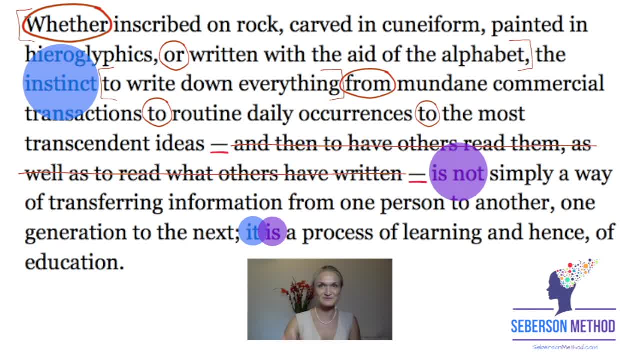 pronoun it refers to, because she also knows. it's really easy for her to lose comprehension if she doesn't know what pronouns refer back to, And then she's going to read the sentence and then she will see that, whether inscribed on rock, caved in cuneiforms, painted in hieroglyphs, 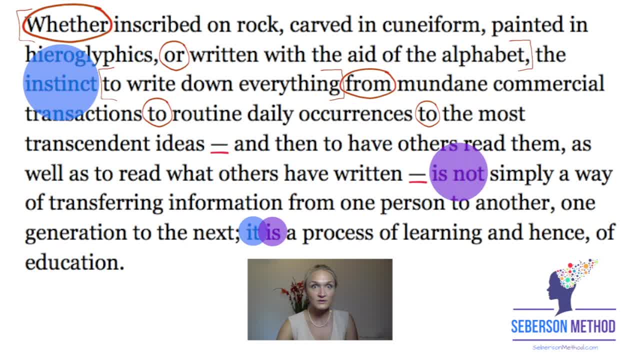 or written in with the aid of the alphabet. all of this is just an opener. The instinct to do what? To write down everything, everything from mundane commercial transactions to routine daily occurrences, to the most transcendent ideas, and then to have others read them, as well as to read what others have written, is not simply a way of transferring. 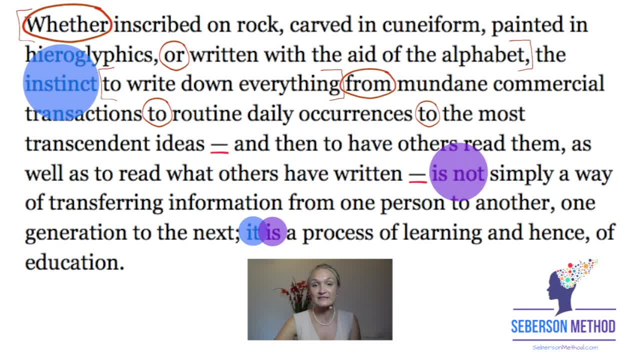 information from one person to another, one generation to the next, next idea. it is a process of learning and hence of education, And it, in the sense, refers back to your instinct to writing everything down. So what the sentence is saying is the instinct to write everything.